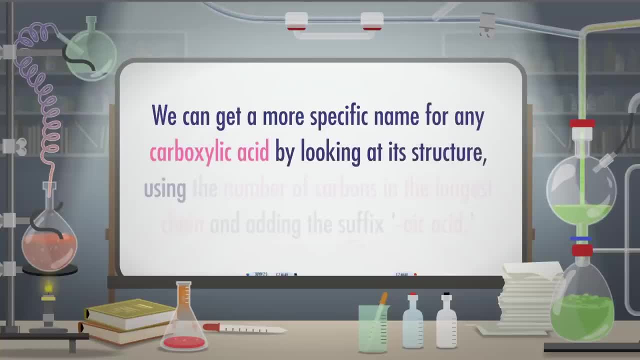 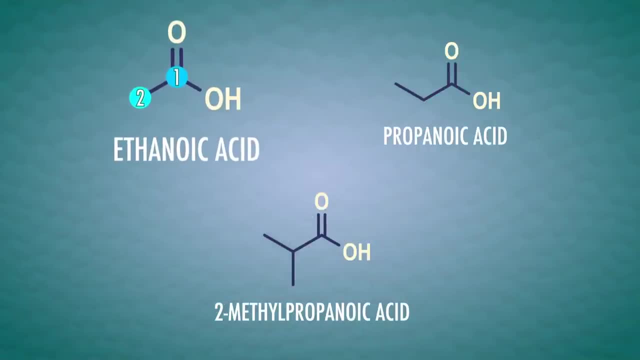 We can get a more specific name for any carboxylic acid by looking at its structure, using the number of carbons in the longest chain and adding the suffix oic acid. A carboxylic acid with two carbons is ethanoic acid. 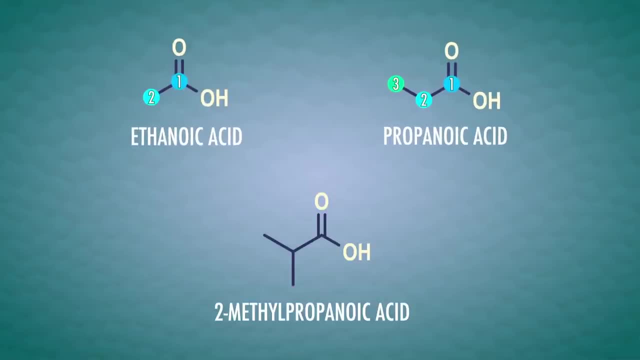 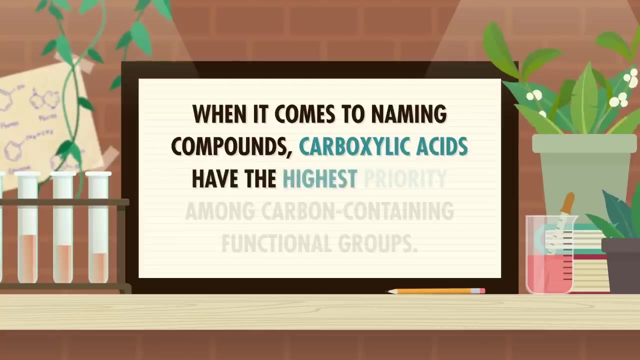 a carboxylic acid with three carbons is propanoic acid and so on. So in the previous reaction we made two methyl propanoic acid. When it comes to naming compounds, carboxylic acids have the highest priority. 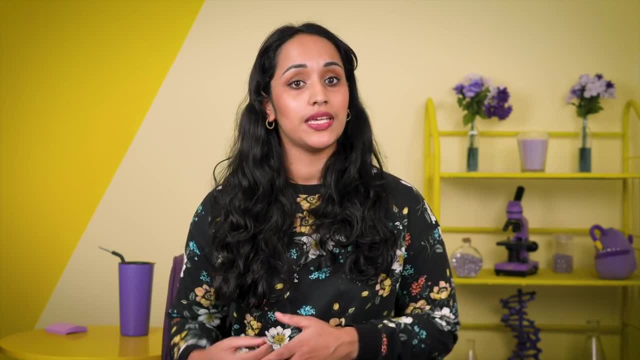 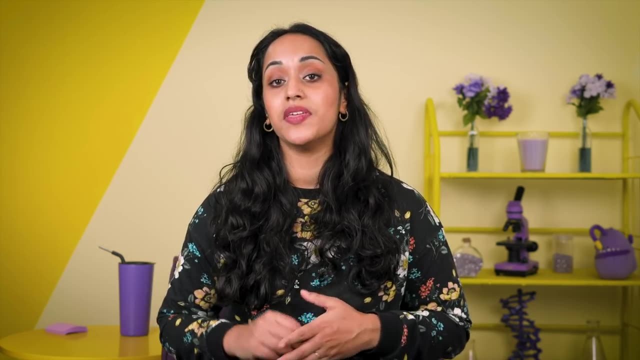 when containing functional groups. So say, we have a molecule containing both a ketone and a carboxylic acid group, The carboxylic acid forms the base name, We assign the carboxylic acid carbon the number one, and the ketone gets a prefix. 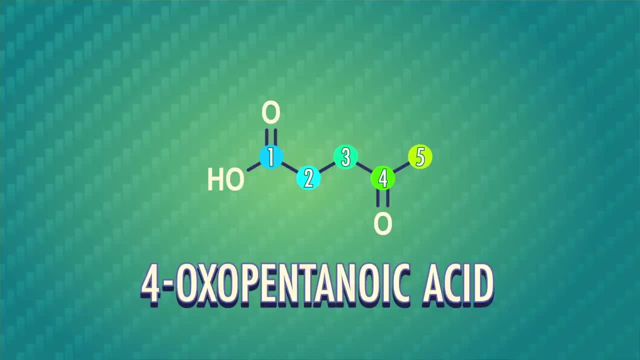 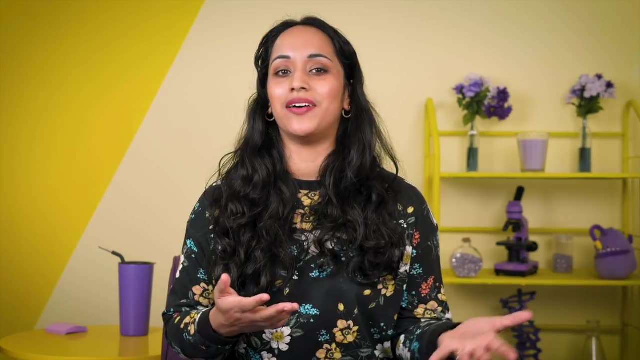 An example of this is 4-oxopentanoic acid, also known as lebulinic acid, a compound used as the starting point for the synthesis of some pharmaceuticals and industrial chemicals. This compound, like many we've mentioned, has a systematic IUPAC name and a common name. 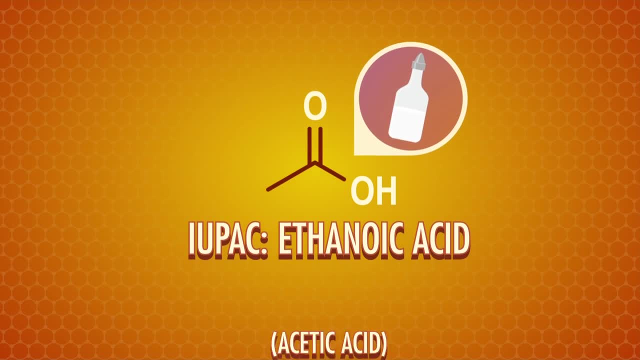 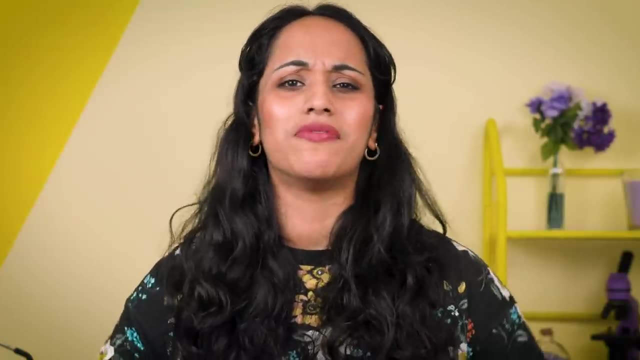 ethanoic acid. the acid in vinegar has the common name acetic acid. As you'd expect from all these names, carboxylic acids are acidic. If they have, oh, about four carbons or fewer, they can dissolve in water. 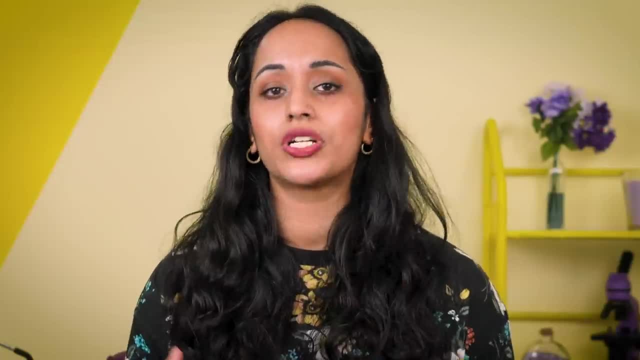 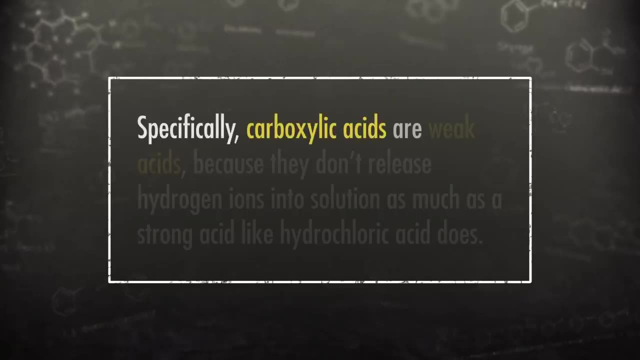 The hydrogen in the COOH part of the structure will be partially ionized, forming a hydrogen ion and leaving behind a carboxylate ion. Specifically, carboxylic acids are weak acids because they don't release hydrogen ions into solution as much as a strong acid. 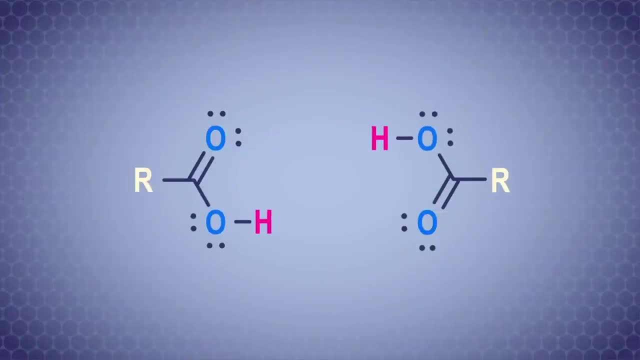 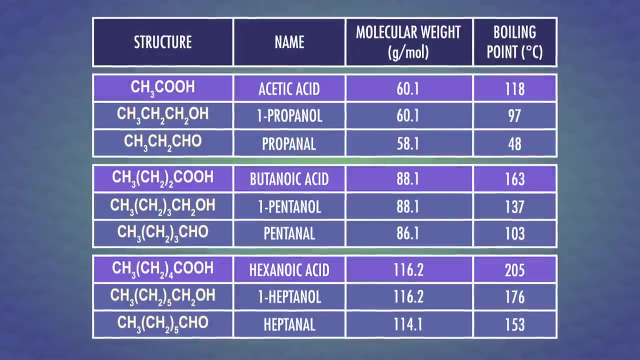 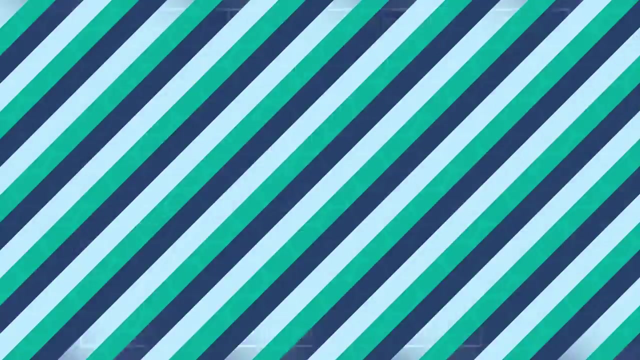 like hydrogen sulfate does. The COOH part of these structures allows intermolecular hydrogen bonds to form between two acid molecules or an acid in water. So carboxylic acids have high boiling points and all those with fewer than 10 carbons in a straight chain are liquids at room temperature. 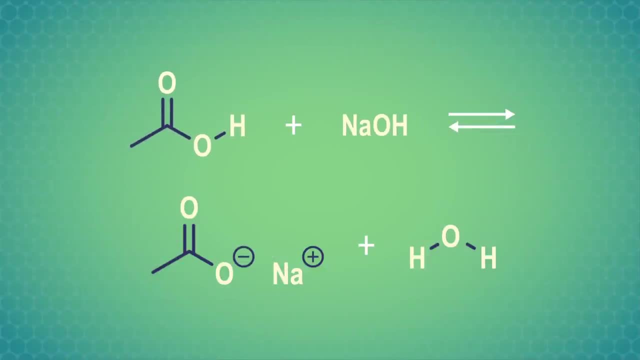 We can react shorter-chain carboxylic acids with sodium or potassium hydroxide to form water-soluble salts too. The hydroxide ion grabs the proton from the carboxylic acid group, forming water and leaving a carboxylate ion behind. 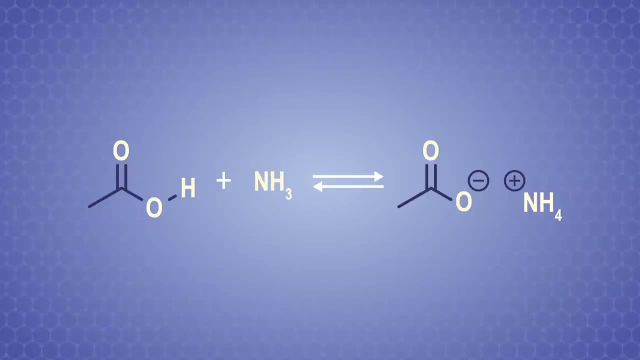 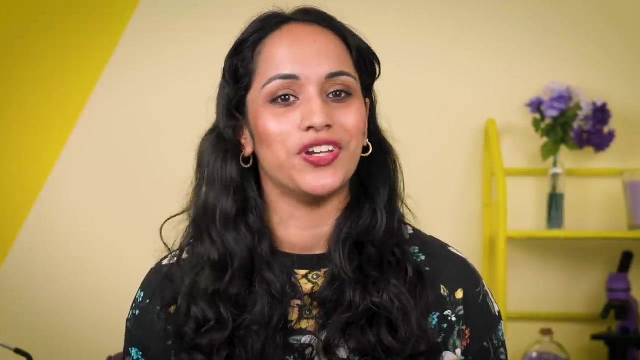 In fact, even weak bases like ammonia can pull off a hydrogen ion and form a carboxylate ion. As we know from earlier episodes, both hydroxide ions and ammonia are good nucleophiles, Which actually highlights an issue that can come up in the lab. Most basic nucleophiles tend to deprotonate carboxylic acids. So, unlike aldehydes and ketones, we can't just use a nucleophile to add groups to the carbonyl carbon. here We'll have to get a little more creative with our chemistry. 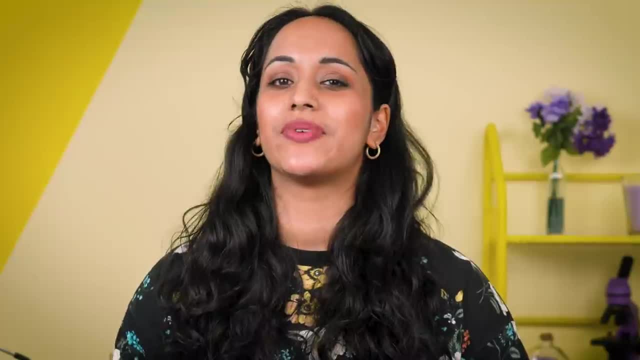 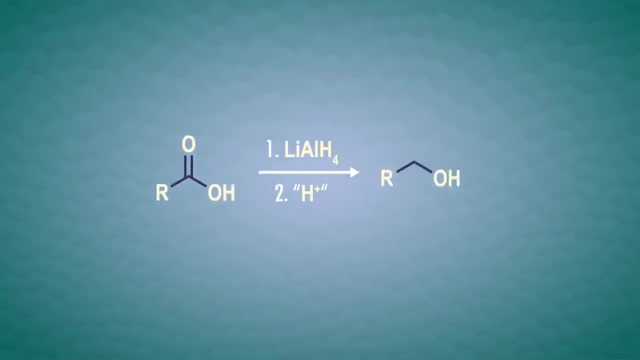 Before we tackle that problem, though, let's look at some other reactions Carboxylic acids can undergo. If we want to get back to an alcohol from a carboxylic acid, we can use a reducing agent such as lithium aluminum hydride. 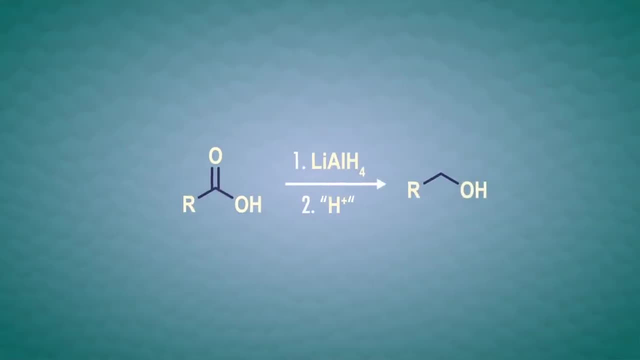 This is a powerful reducing agent. So after the reaction we add a proton source very carefully to react any unreacted lithium aluminum hydride and give our alcohol a proton back. Another way to remove the carboxylic acid group has a very straightforward name. 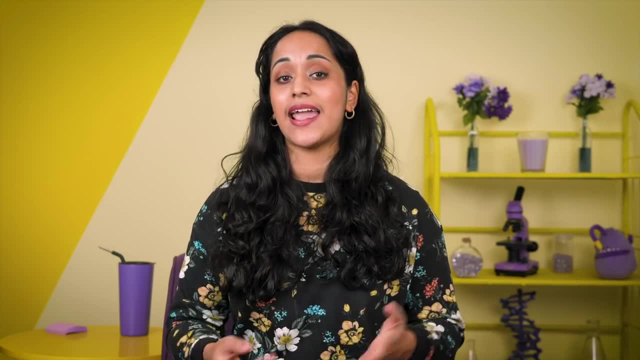 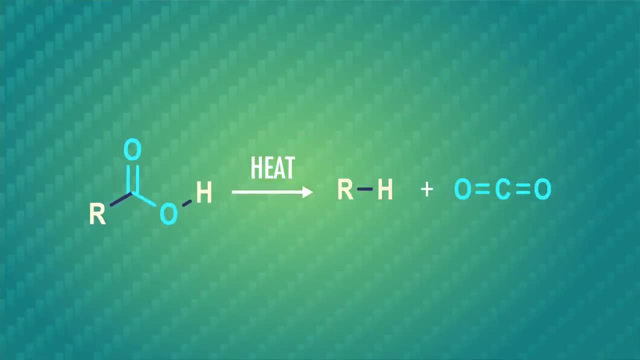 Decarboxylation. This involves heating the carboxylic acid and replaces the carboxylic acid group with a hydrogen atom. So if we heat the heck out of almost any carboxylic acid, we can get it to decarboxylate. 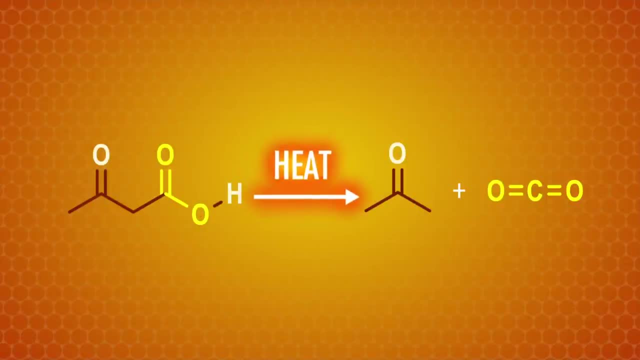 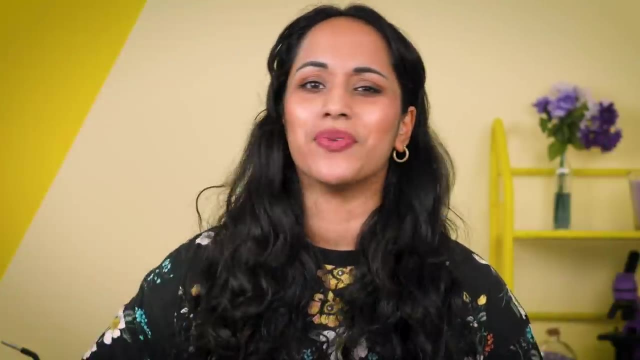 And this reaction happens really easily when you heat compounds that have a carbonyl group- one carbon- away from the carboxylic acid group. However, sometimes you don't want to get rid of the carboxylic acid group entirely, So there are also reactions to convert it to other functional groups. In fact, we can freshen up some of those bad smells by converting carboxylic acids into pleasant-smelling esters by Fischer esterification. This is an acid-catalyzed reaction of a carboxylic acid with an alcohol to form an ester. 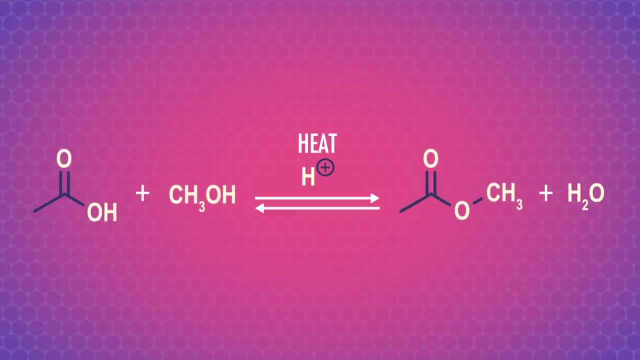 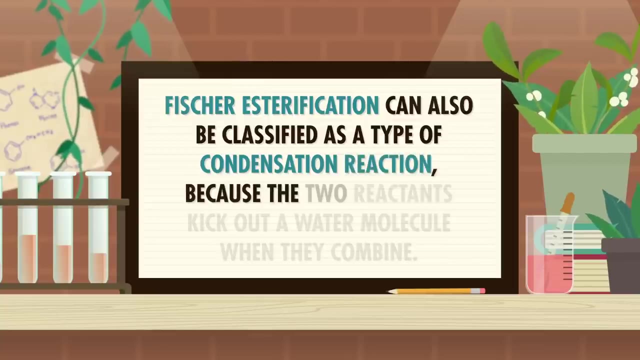 Esters are often key parts of the smells of flowers and fruits and are commonly used in perfumes. Fischer esterification can also be classified as a type of condensation reaction, because the two reactants kick out a water molecule when they combine. 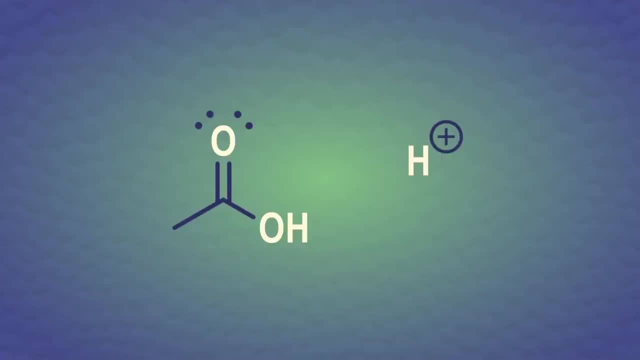 To get more specific: first, the carbonyl oxygen grabs a proton from the acid catalyst. Next, the lone pair on the alcohol oxide grabs a proton from the acid catalyst. Next, the lone pair on the alcohol oxide grabs a proton from the acid catalyst. 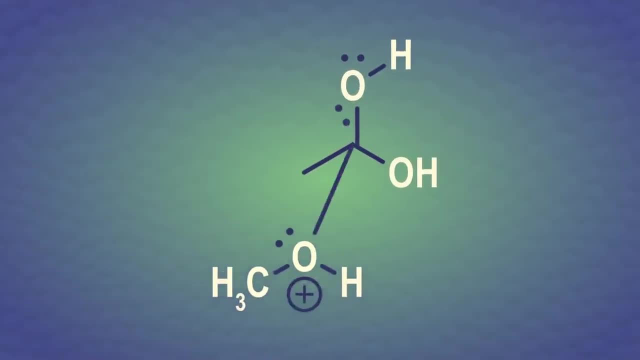 Next, the lone pair on the alcohol oxide grabs a proton from the acid catalyst. The lone pair on the alcohol oxygen acts as a nucleophile, attacking the carbonyl carbon. Another alcohol molecule swoops in, deprotonating the hydrogen from the 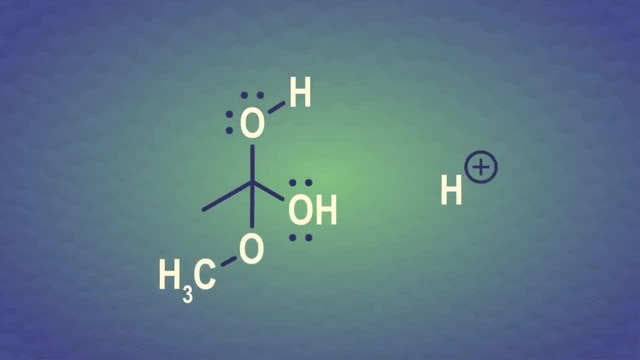 oxonium ion in that one-two punch of attack. then deprotonation we're getting familiar with. The OH group on the carboxylic acid finds a hydrogen ion from the acid catalyst which makes water a good leaving group, With a little help from the neighboring oxygen atom in the molecule the water leaves. 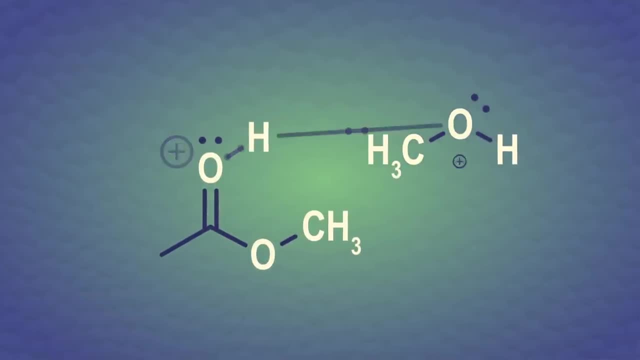 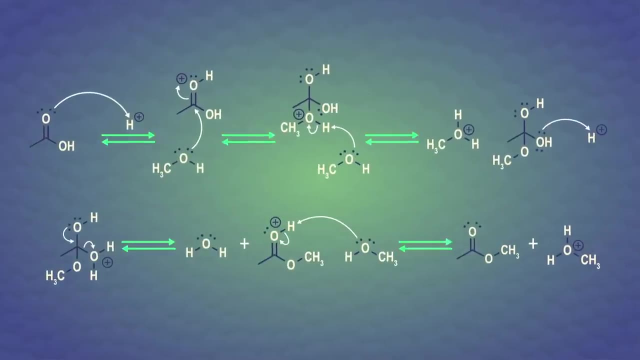 And finally, another alcohol molecule from solution grabs the extra hydrogen on the carbonyl oxygen, giving us an ester as our final product. All of these steps are reversible, so the product isn't formed super efficiently, But never fear, Le Chatelier is here. 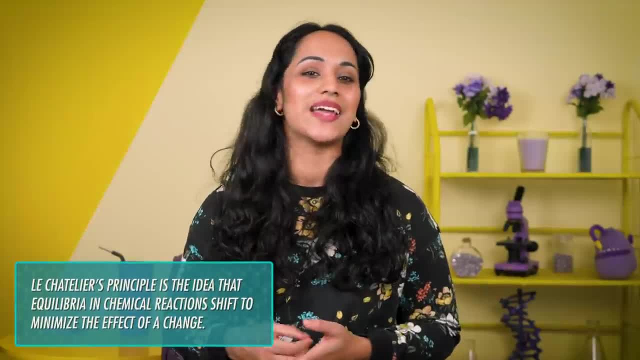 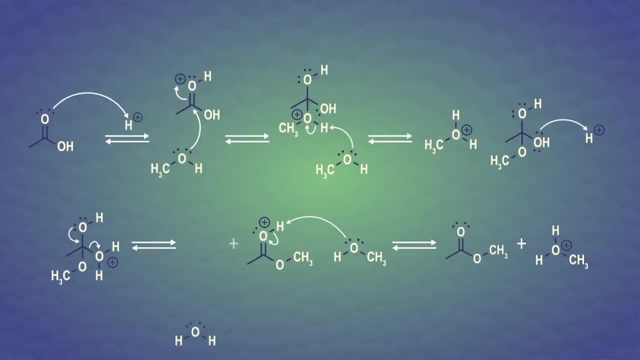 We have the power to adjust the equilibrium of chemical reactions. Specifically, if we remove one of the products along the way, we can push the reaction forward In a lab. removing the water as it forms using a special piece of equipment increases our yield of the ester. 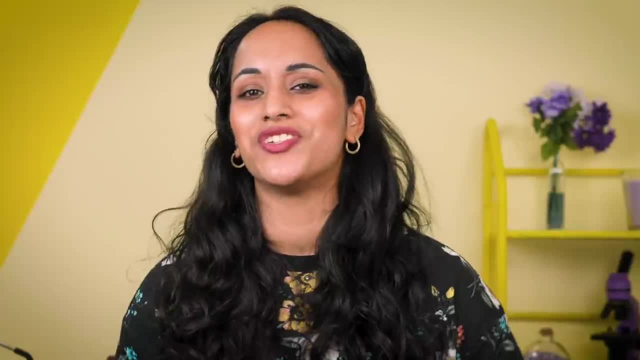 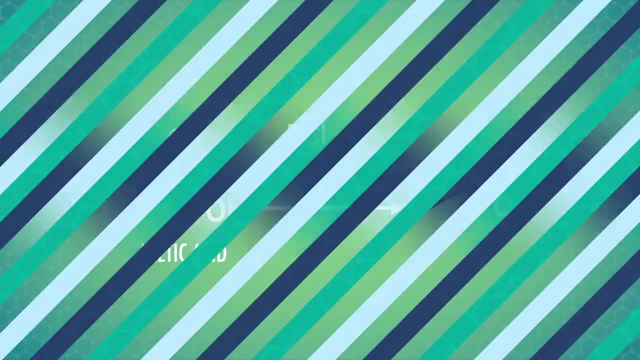 Speaking of tricky lab situations, How about that problem? we mentioned earlier The issue of nucleophiles deprotonating carboxylic acids. instead of attacking the carbonyl carbon To solve this problem, we can convert the carboxylic acid to a more reactive functional group. 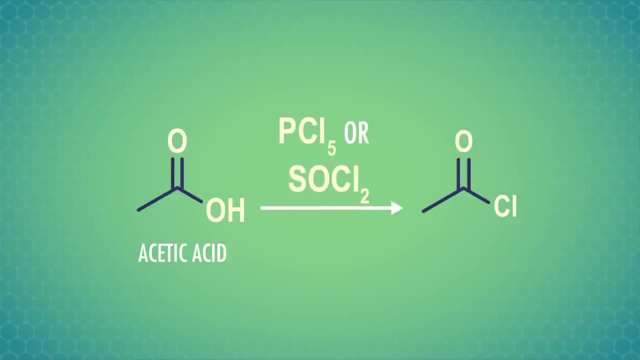 an acid chloride using either phosphorus pentachloride or thionyl chloride, And let's just go with phosphorus pentachloride as our example. The reaction starts when the lone pair of electrons on the carbonyl oxygen forms a bond with the phosphorus atom, with a little help from the other oxygen in the molecule. 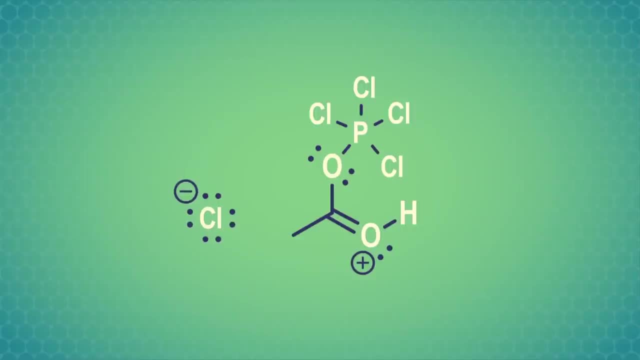 And kicks a chloride ion off of phosphorus pentachloride. The chloride ion we kicked out in the previous step swoops back and attacks the carbonyl carbon. Then a very stable double bond forms between the phosphorus and this oxygen. 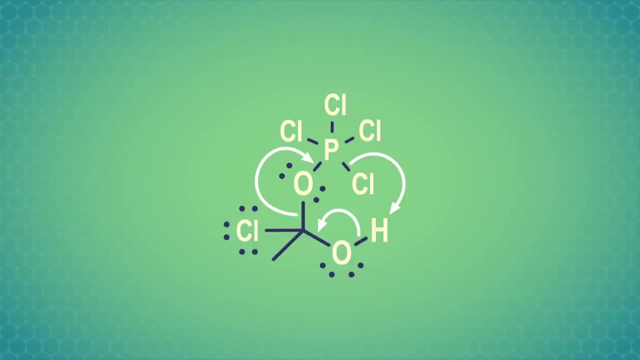 This double bond is a big part of why this reaction happens this way, just like we saw in the Wittig reaction in episode 28.. Specifically, with the formation of this bond, we lose chloride as a leaving group which pulls off the nearby hydrogen to reform our carbon-oxygen double bond. 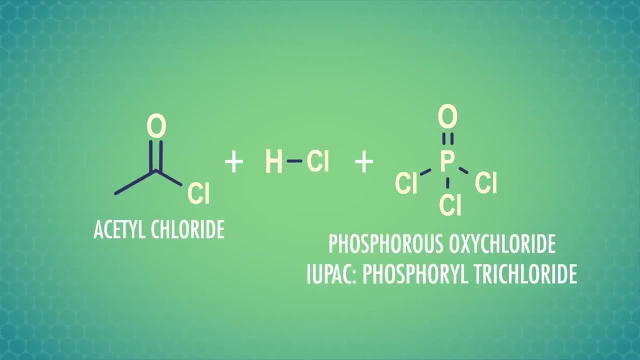 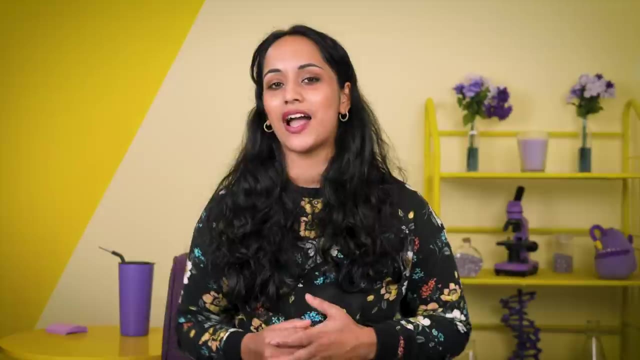 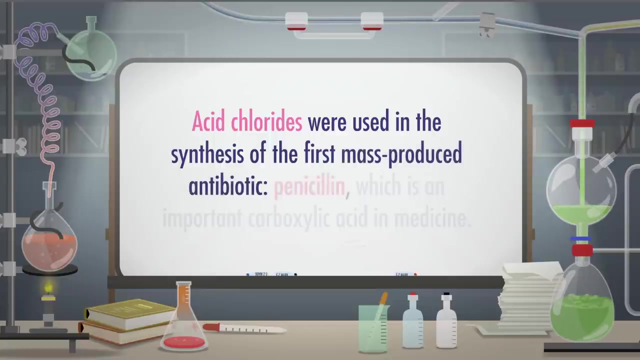 This gives us the acid chloride With hydrochloric acid and phosphorus oxychloride as the other products. Acid chlorides, along with other carboxylic acid derivatives, are involved in many useful reactions in organic chemistry. In fact, acid chlorides were used in the synthesis of the first mass-produced antibiotic. 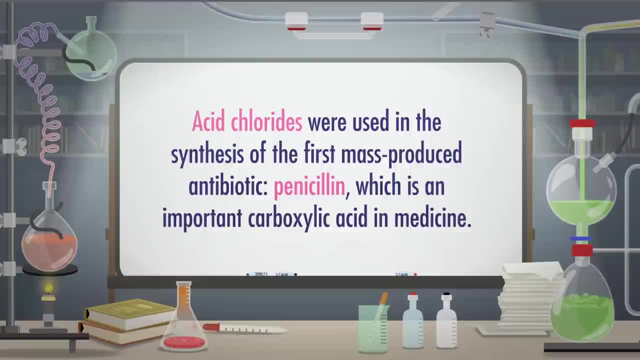 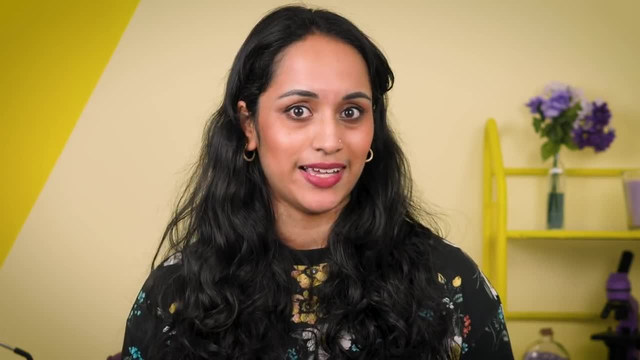 penicillin, which is an important carboxylic acid in medicine. Throughout the rest of the Crash Course Organic Chemistry series, we'll apply many of the reactions we learned to explore the chemical synthesis of penicillin. But penicillin was an accidental discovery. 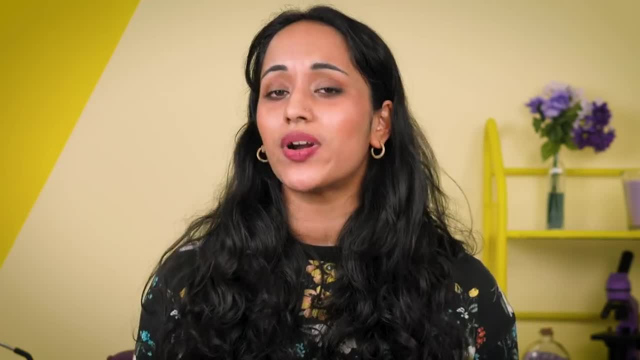 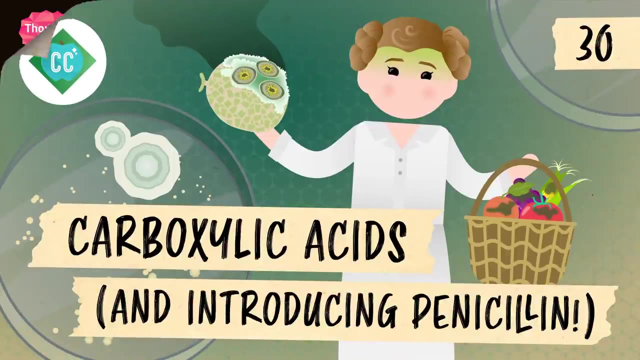 Not a medicine dreamed up by humans, And the story of this compound is much more complicated than just one scientist making a lucky discovery in 1928. Let's head to the Thought Bubble to learn more. Returning to his lab after a summer holiday, the microbiologist Alexander Fleming discovered: 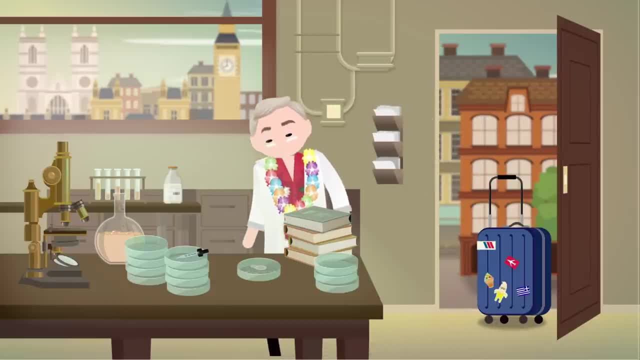 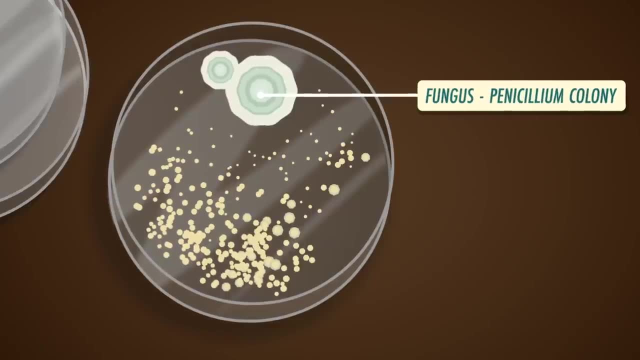 that one of his petri dishes of bacteria had been unintentionally left out on a bench. Spores of a fungus had blown into the lab and contaminated the dish, and the temperatures had been perfect to encourage both the fungus and the bacteria to leave. 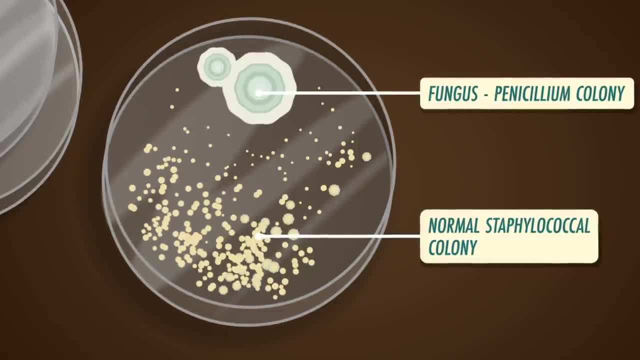 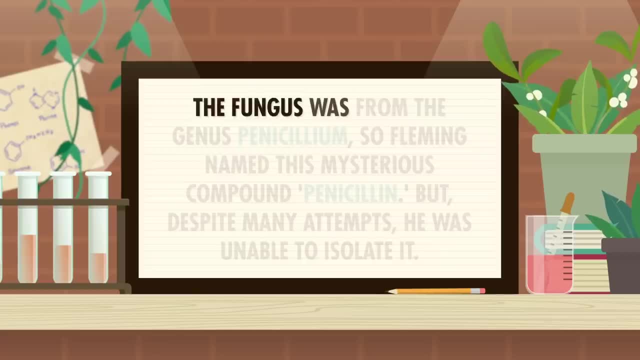 So what's next? The bacteria had grown, But wherever the fungus had grown, the bacteria were absent. Fleming realized that the fungus made a chemical compound that killed the bacteria. The fungus was from the genus Penicillium, So Fleming named this mysterious compound penicillin. 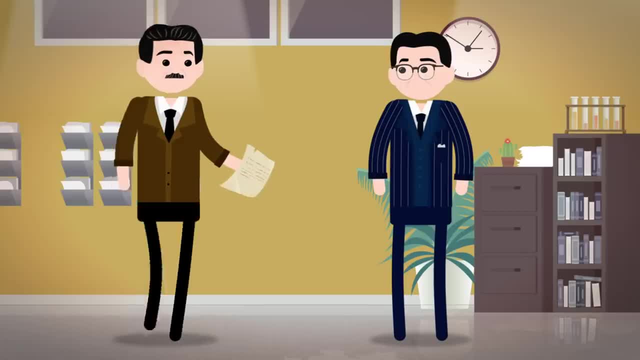 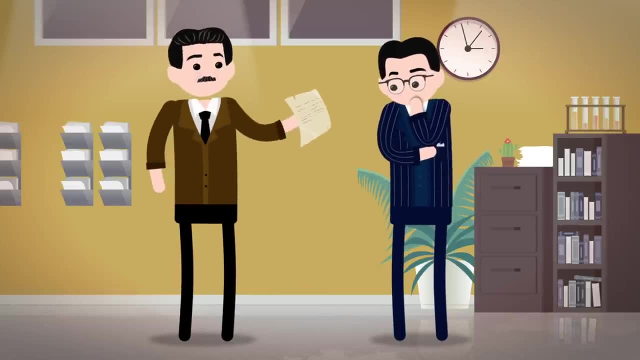 But despite many attempts he was unable to isolate it. At Oxford University a biochemist named Ernst Chain found Fleming's publication on penicillin and suggested to his supervisor, Howard Florey, that they try to isolate it. Penicillin was eventually isolated and purified in 1941. 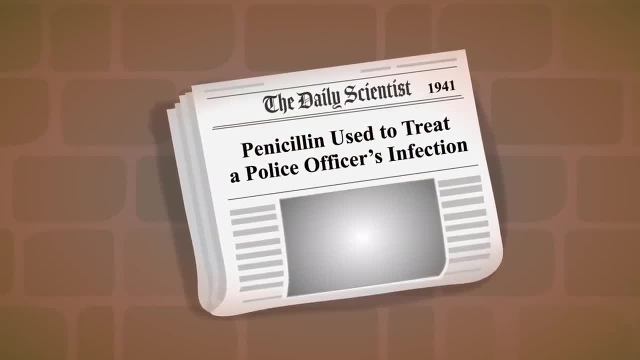 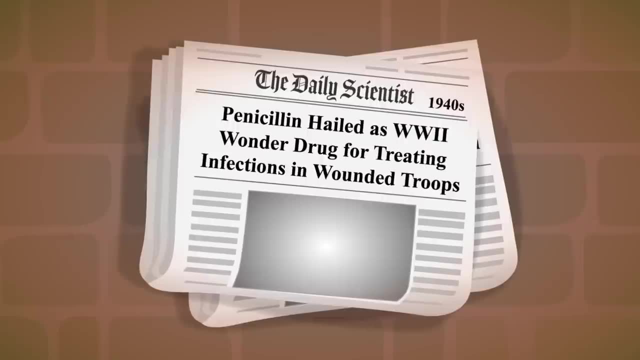 That same year, penicillin was first used to treat an infection in a police officer. It was later hailed as a wonder drug during World War II for its ability to combat infections in wounded troops. But there was still a huge unsolved problem in the early 1940s – the low yield of penicillin from the mold. 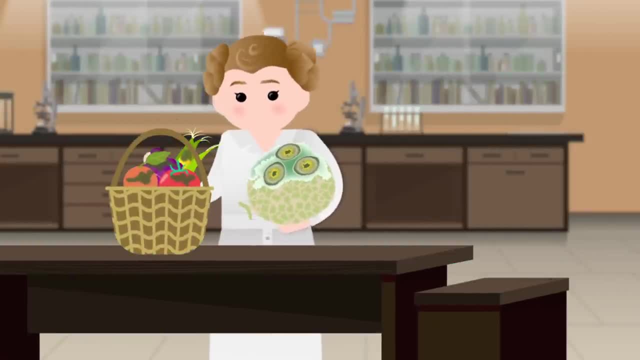 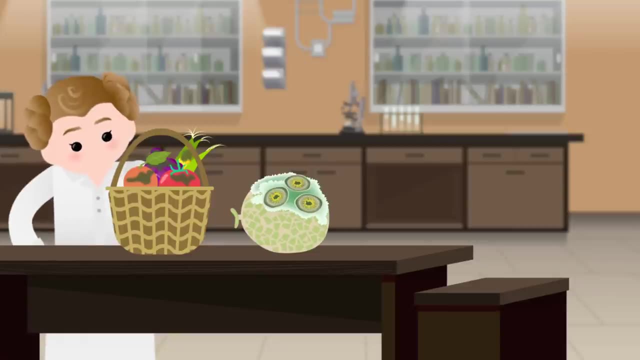 In 1943, a bacteriologist named Mary Hunt made a breakthrough while working at the US Department of Agriculture's Northern Regional Research Laboratory in Peoria, Illinois, Illinois. Nicknamed Moldy Mary, she hunted down moldy fruits and vegetables to test for the presence. 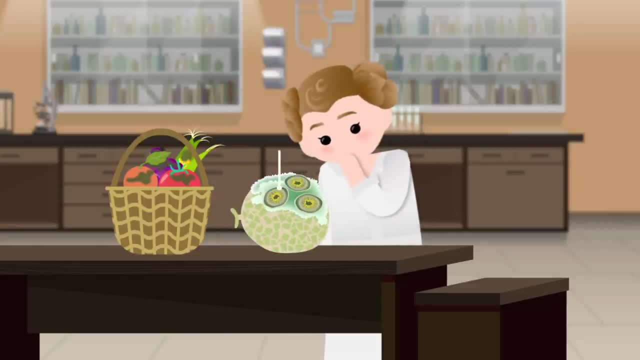 of penicillin. in the lab, A spoiled cantaloupe melon had a fungus, Penicillium chrysogenum, that produced 200 times more penicillin than the fungus that Fleming stumbled upon, making mass production possible. 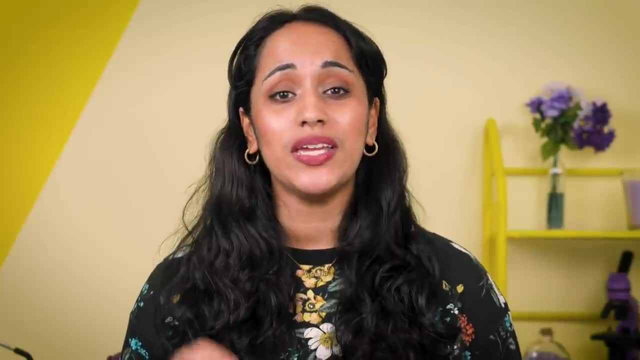 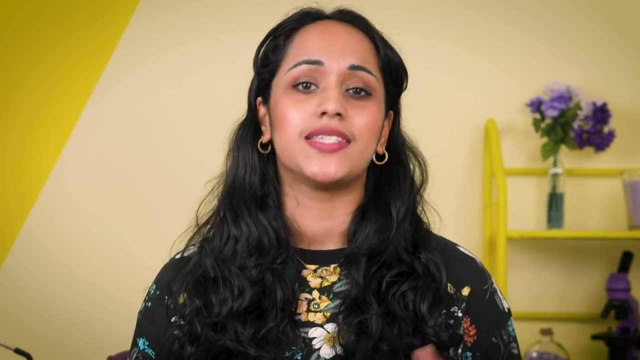 Thanks, Thought Bubble. Since Mary Hunt's cantaloupe discovery we've learned a lot more. Like the, penicillins are actually a family of compounds with different potencies and ways to administer the medicine. The penicillin that Fleming discovered and Chain and Florey isolated and even won a 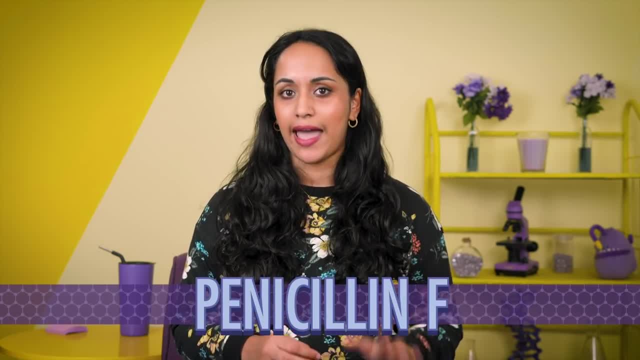 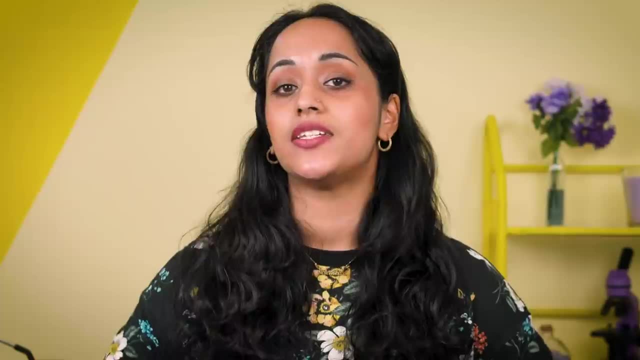 Nobel Prize for in 1945, was penicillin F. The stuff that was produced from Hunt's spoiled cantaloupe melon was penicillin G. In later episodes we'll be looking at Dr John C Sheehan's synthesis of penicillin.